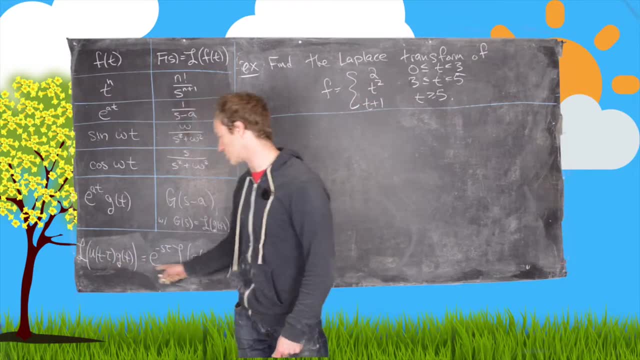 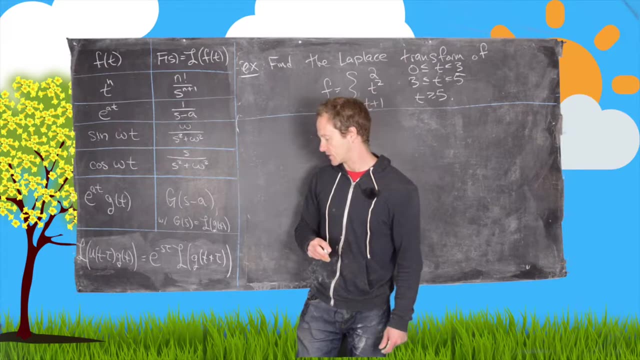 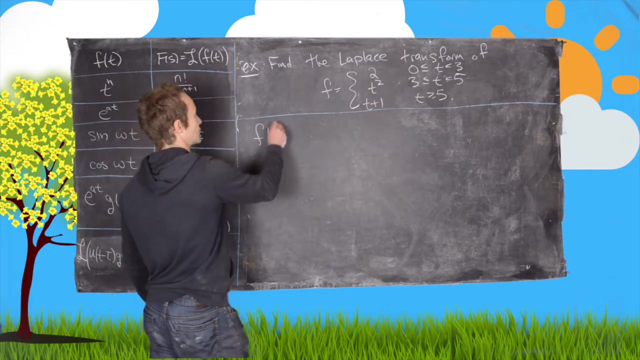 So we have the Laplace transformation of this shifted unit step function times a. function g is e to the minus s tau, and then this Laplace transformation of this function g, evaluated at t plus tau. Okay, so let's see what we can do here. So the first thing to do is to rewrite this piecewise function using the unit step function. 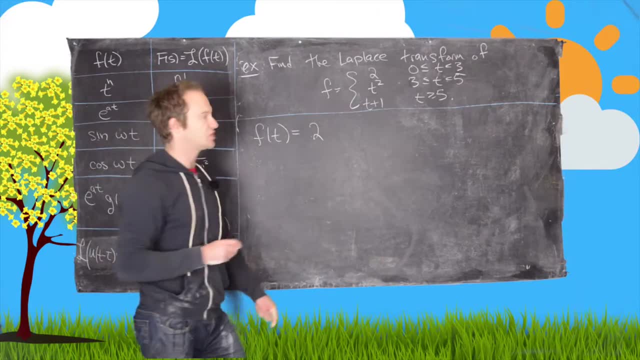 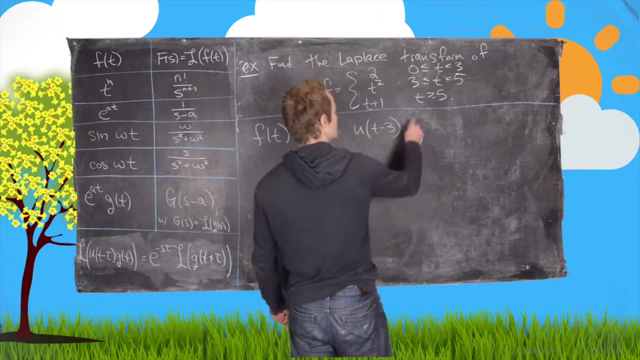 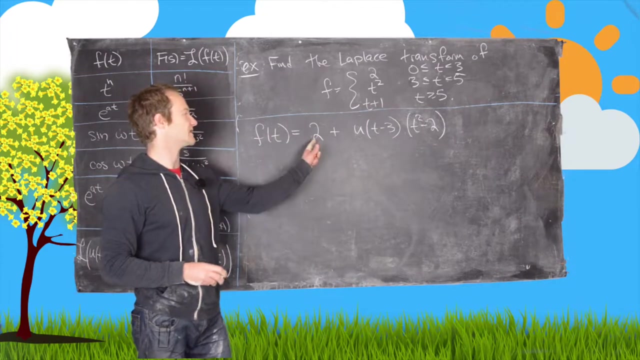 And we can do that as follows. So this is equal to 2 plus u of t, minus 3 times t squared minus 2.. So maybe that's the first thing to notice is that notice 2, this will be good for all times. 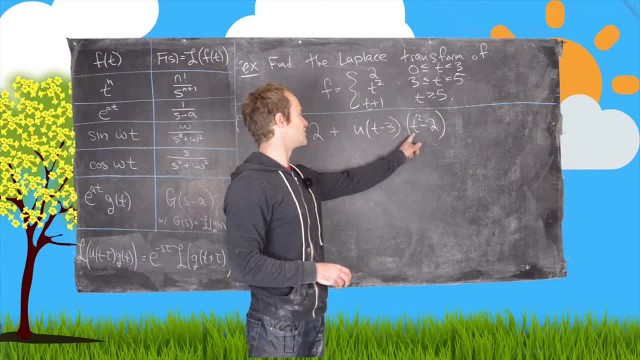 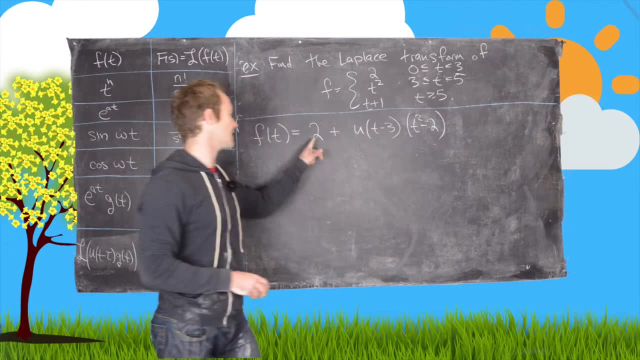 So we have t bigger than or equal to 0, but now we want it just to be equal to t squared if we're bigger than or equal to 3.. So we include a t squared here, but then we include a negative 2 to counteract this. 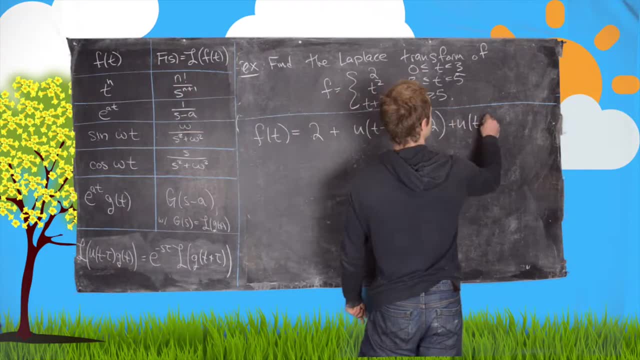 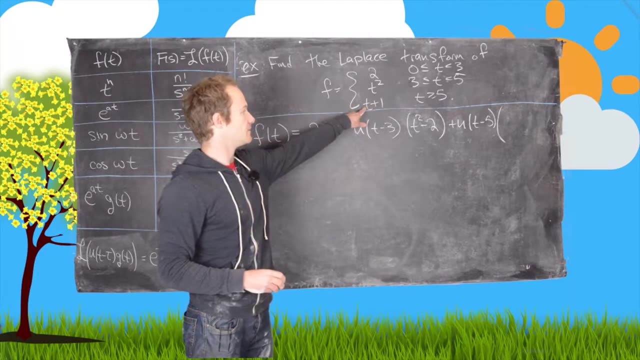 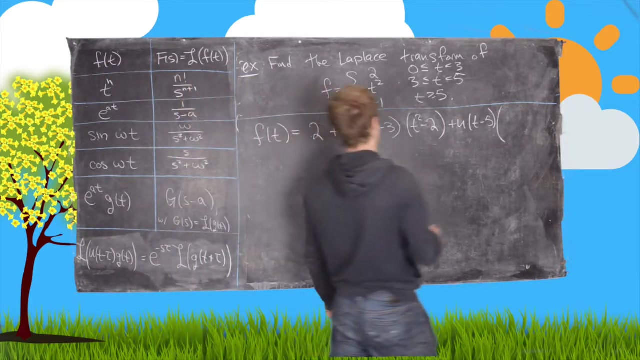 And then we have: this is plus u of t, minus 5 times. and now here we're going to have to do t plus 1, and then it's going to be minus this, Yeah, and then we're good. So let's see what we get for that. 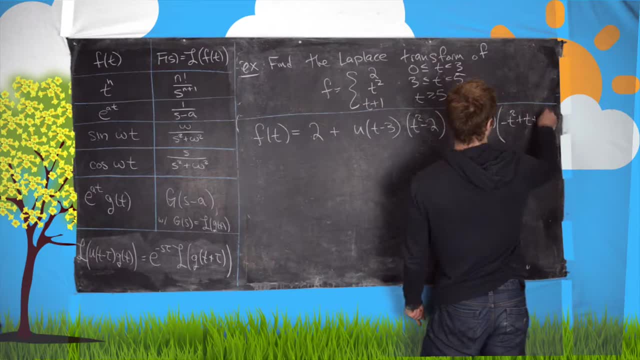 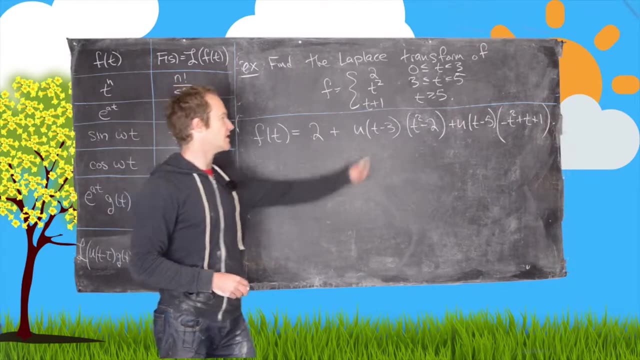 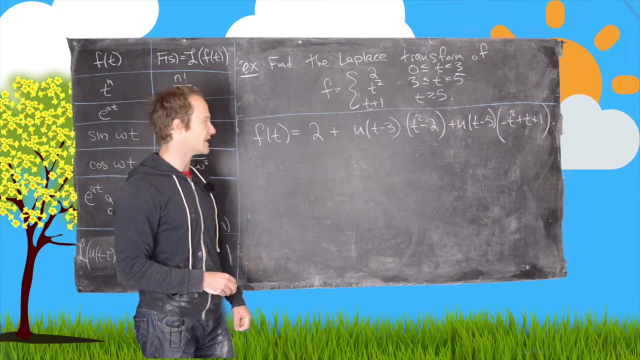 So we get minus t squared, plus t plus 1.. Okay, so now let's make sure this makes sense. So if we're between 0 and 3, these two unit step functions are 0. so we're okay, Good. And now notice: if we're between 3 and 5, this unit step function gives us 1, this one gives us 0.. 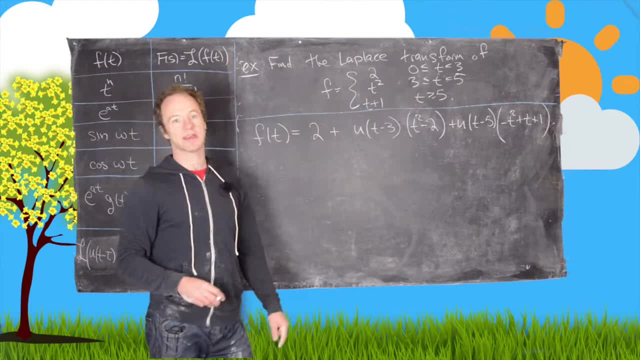 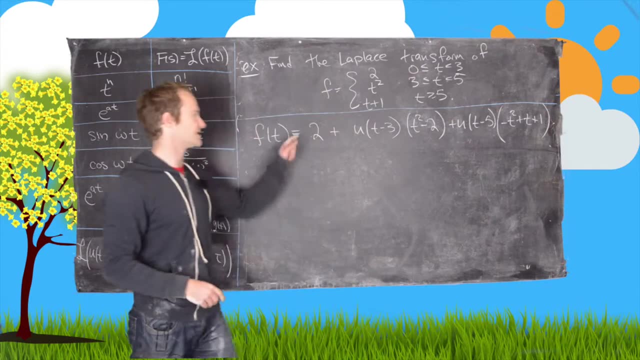 And so notice this negative 2 and this 2 cancel each other out, and we're just left with t squared. Okay, So now we're going to apply this rule involving the unit step function to simplify these. So let's see what we get. 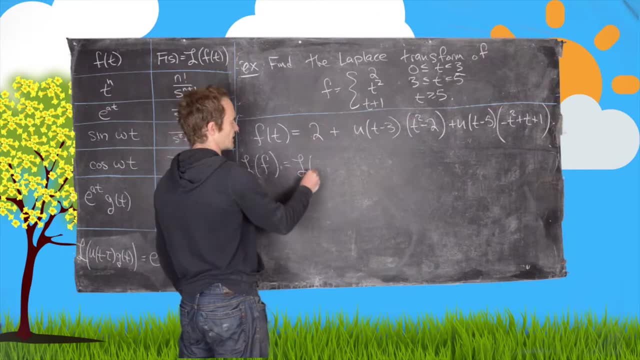 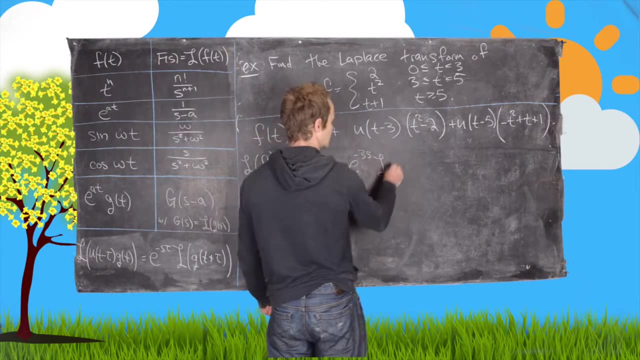 So this is going to be: the Laplace transform of f equals the Laplace transform of 2 plus now, look, this is going to be e to the minus 3s times, the Laplace transform of t plus 3, squared minus 2.. 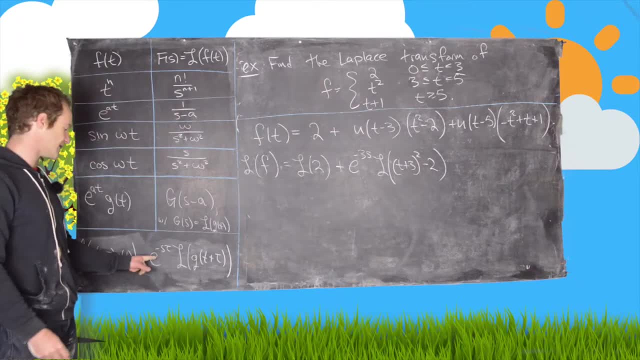 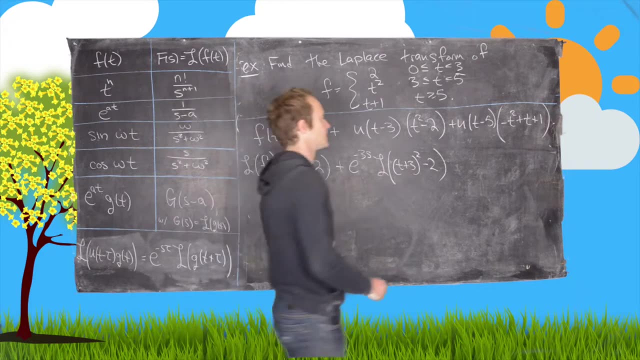 And so that's using this rule. So notice, we have e to the minus s tau and g of t plus tau. So we have: it looks like it's 2.. It looks like it's going in 2 directions here, And so then here we're going to have plus e to the minus 5s. 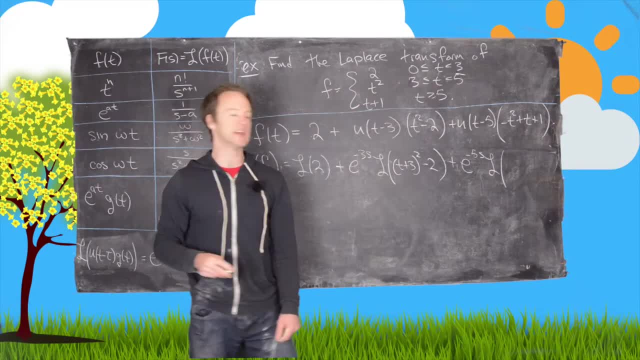 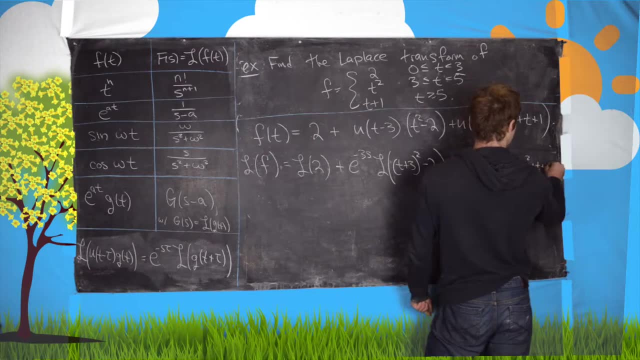 And this is going to be the Laplace transform of this, where we replace t with t plus 5.. So that's going to be minus t plus 5, quantity squared plus t plus 5 plus 1.. Okay, great, So now we're ready to do some simplification. 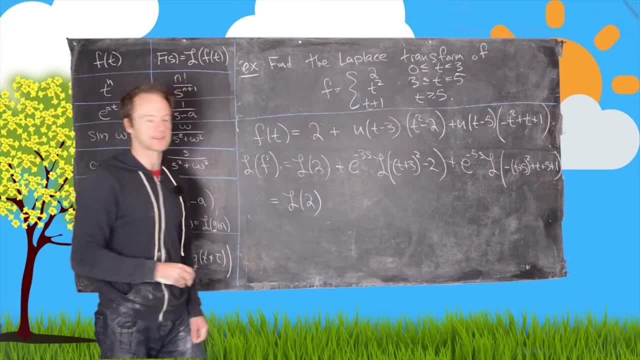 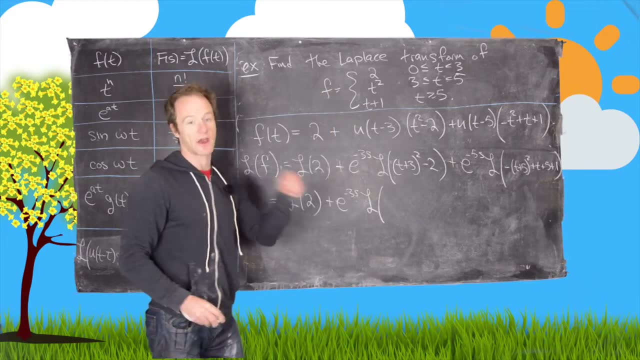 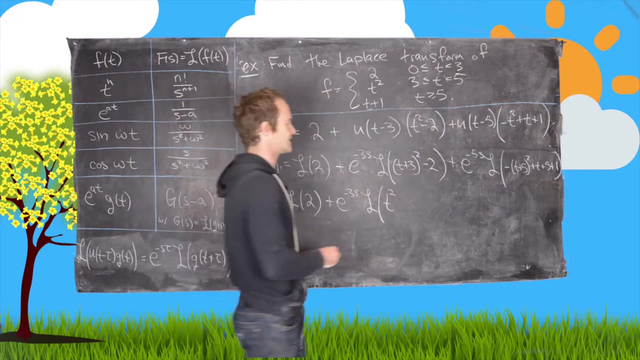 So notice, this is the Laplace transformation of 2.. I won't do that simplification yet. And then plus e to the minus 3s, the Laplace transform of: and now I think we can probably do this really quickly. So notice, if we FOIL this out, we get t squared plus 6t, plus 9, minus 2.. 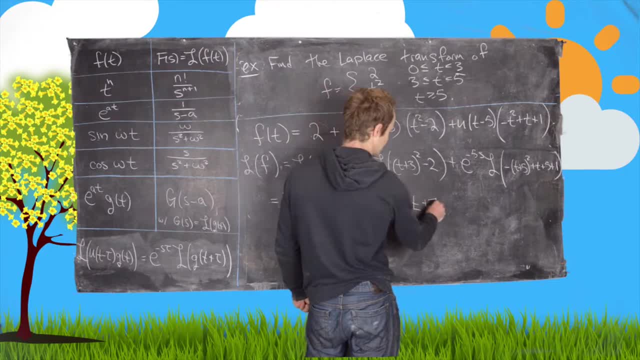 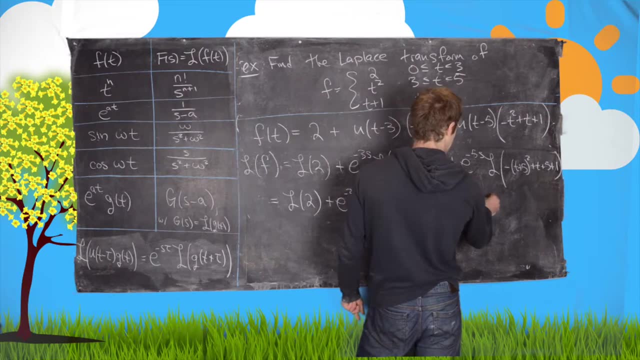 So that's going to be, let's see, plus 7.. Okay, good. And then here we're going to have plus e to the minus 5s, The Laplace transform of. so minus t squared, That's our only t squared term, right. 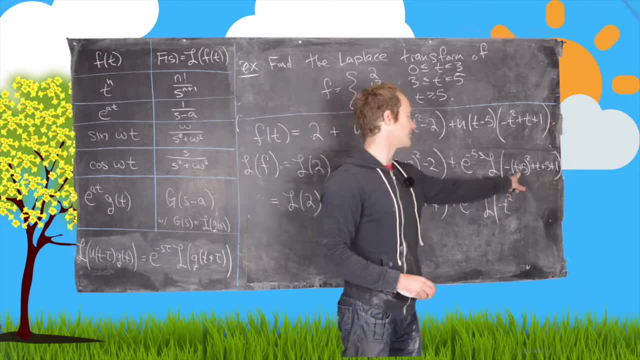 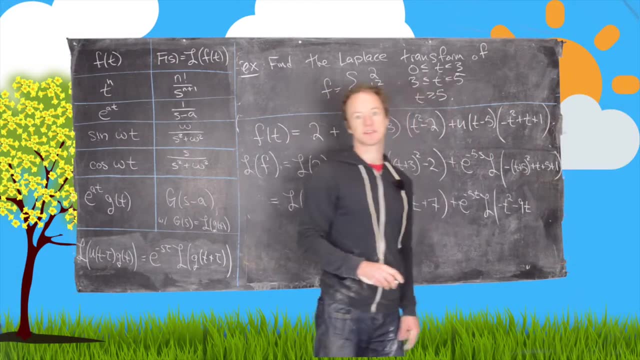 And now we have minus 10t from this term plus t, So that's going to be minus 9t. And we have minus 25 plus 6. So that's going to be minus 21.. Okay, so we've got something like that. 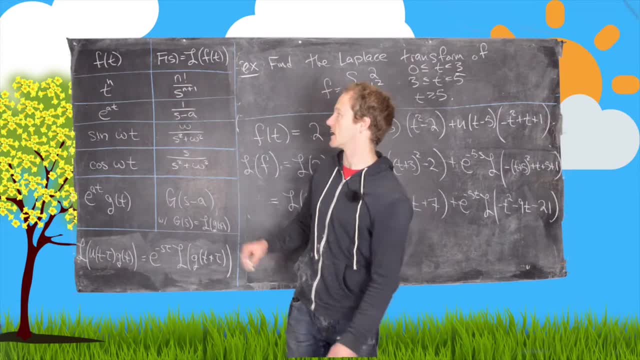 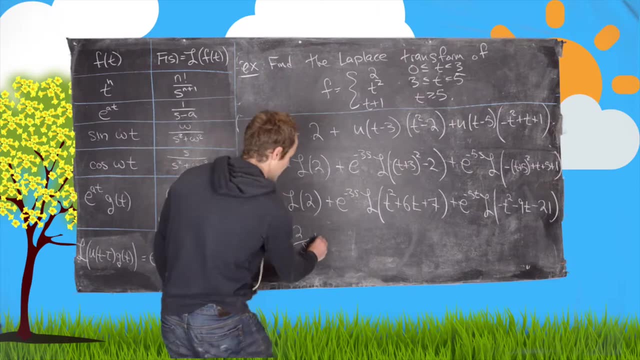 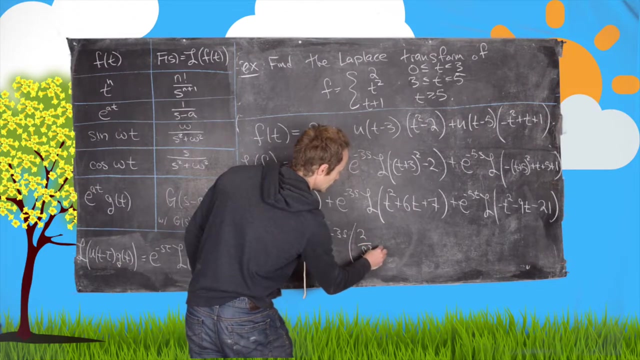 Notice we've got nice polynomials inside of our Laplace transform so we can use this Laplace transform. We've got our first rule, So notice this is going to give us 2 over s plus e to the minus 3s. This is going to give us 2 over s cubed plus 6 over s squared, plus 7 over s. 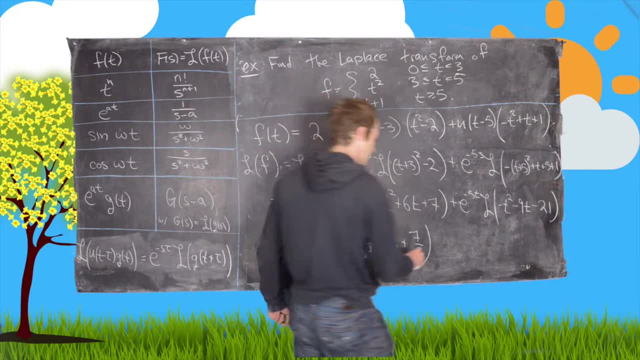 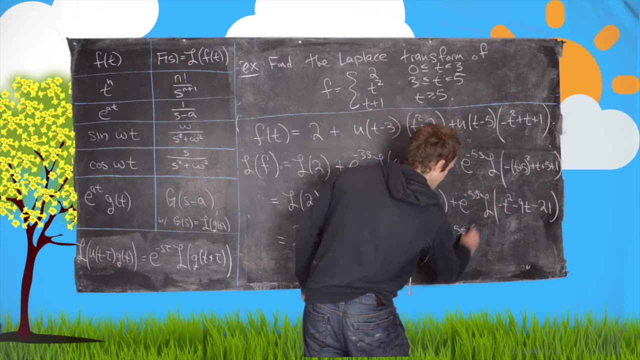 So that's the Laplace transform of this term, And then we'll have: this is plus e to the minus 5s, And then times that's going to give us negative 2 over s cubed, minus 9 over s. squared, minus 21 over s.